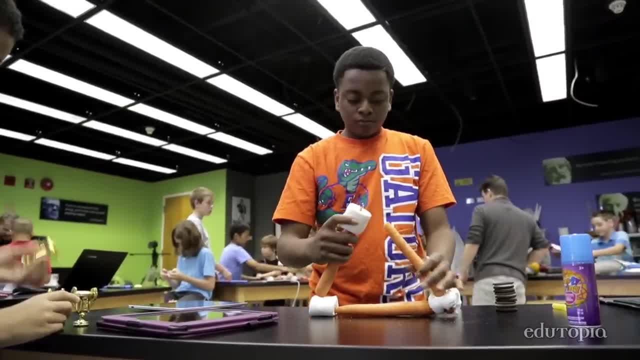 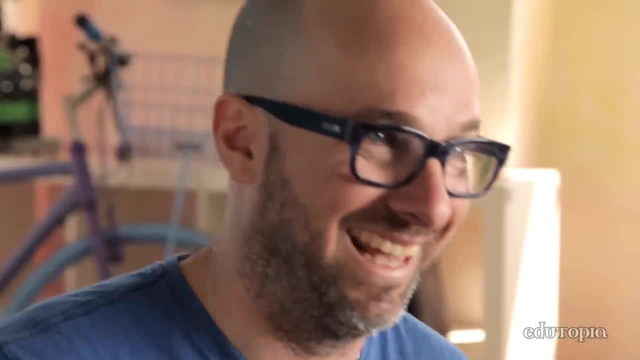 What's the appropriate developmental tools or toys for a 13-year-old to learn, share, iterate flourish. mess up, get excited. I have a mirror triangle, A linen towel with flowers, So you call it blocks. Yeah, Great. 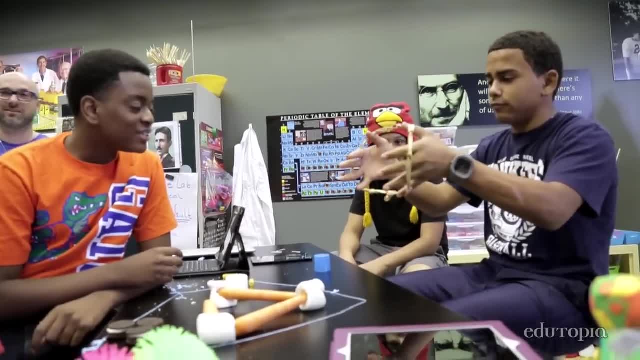 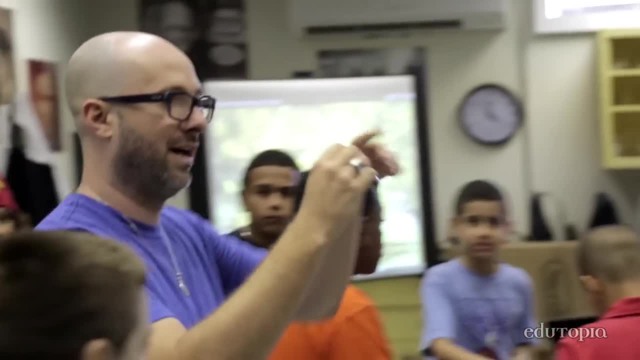 I want someone, as soon as possible, to have a successful experience with something open-ended, so that they can look back and say to themselves: I have accomplished whatever it is we're trying to get. If I touch one side of the circuit and then the other side, it squeaks okay. 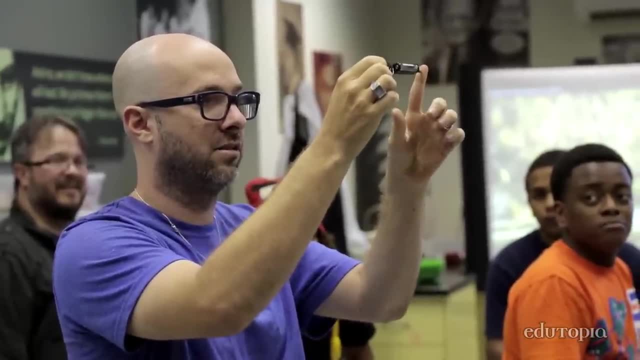 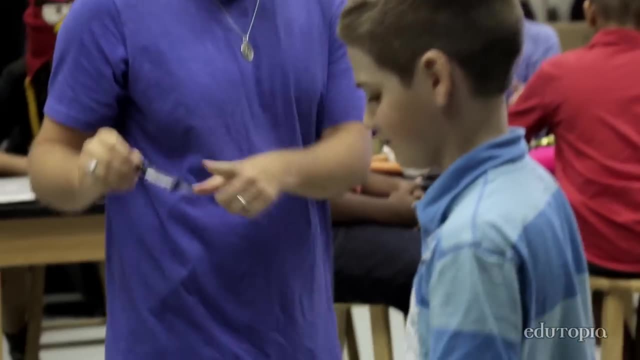 And if I touch it harder, it squeaks higher, And if I touch it less, it squeaks lower. Let's make a little instrument out of this. The simplest instrument you can make is with two people, The way I believe people learn. 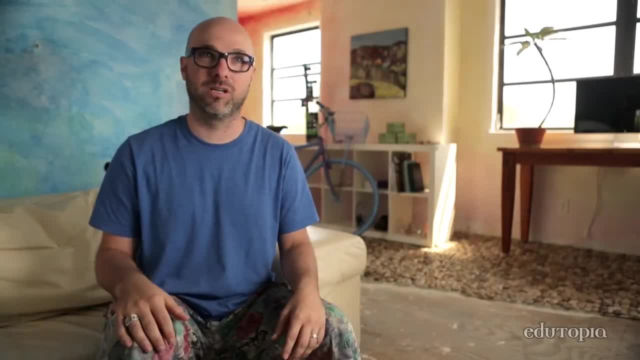 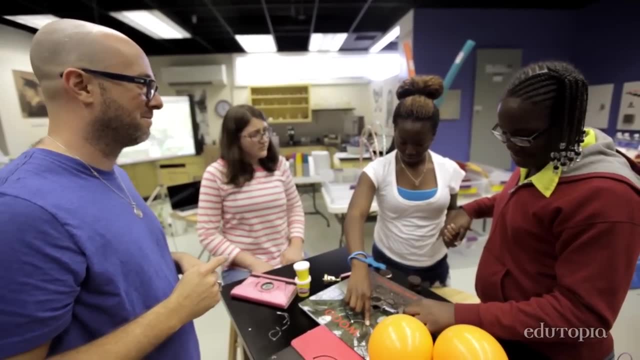 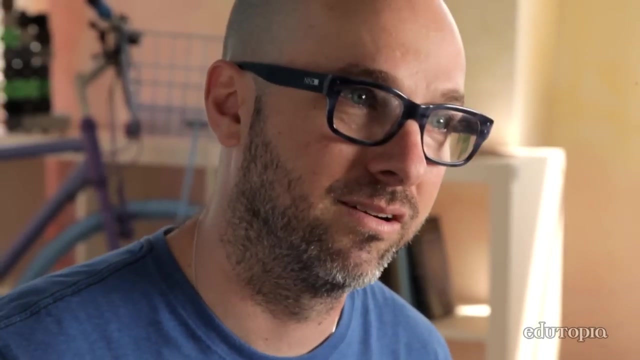 is by carrying out their own processes in the physical world. Hold her hand Now. Yeah, there you go. And now hold tighter, There you go. Yep, I'm only going to teach people by creating a situation where people can then carry out meaningful projects. 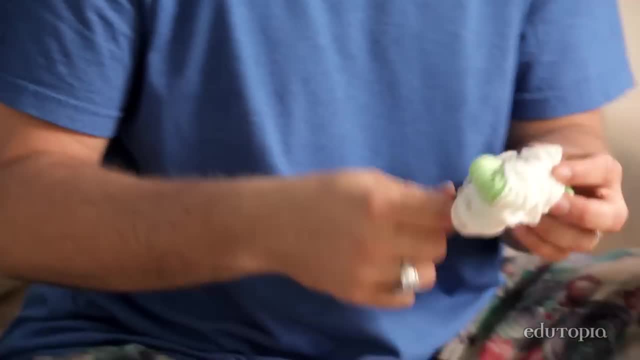 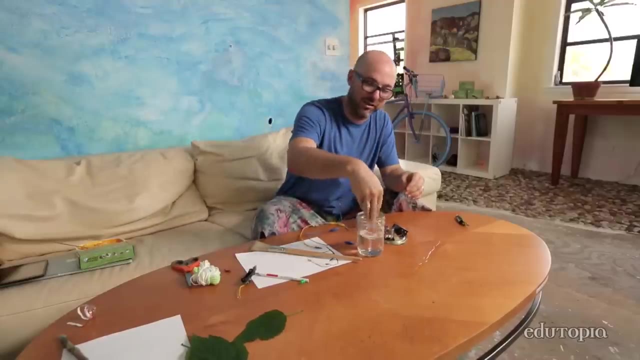 Let's show how you can invent with a circuit like this. Let's take a piece of string. This is just regular yarn. We can dope the string with a certain type of conductive material, In this case water, so I just dip the string in water. 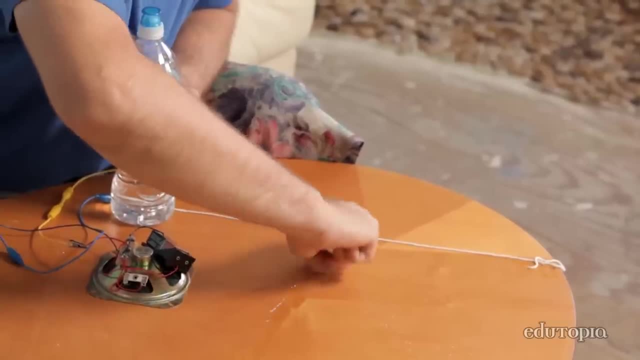 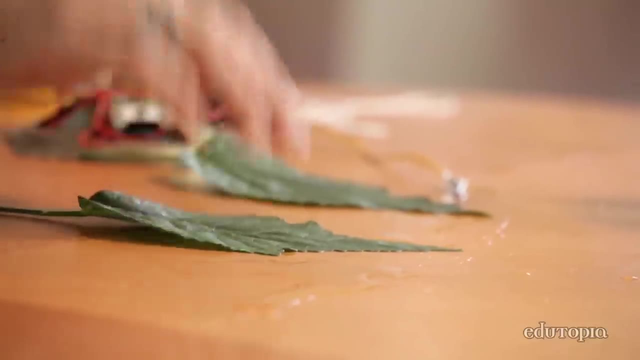 I can even get vibrato Leaves could be like buttons. Everyday objects are in a class of their own And in a sense anything can be cast as an everyday object. But the important thing about everyday objects is that people have familiarity with them. 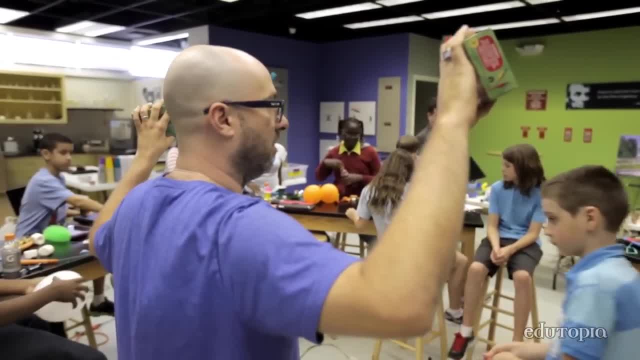 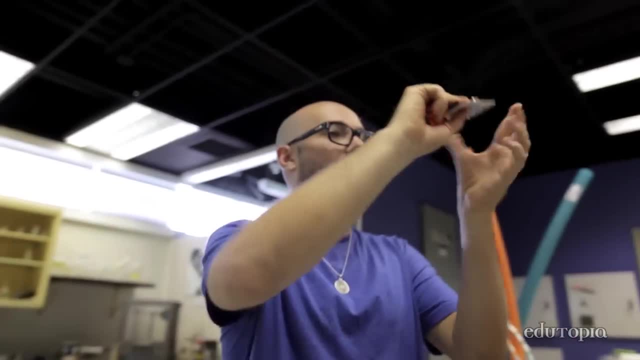 What you do with the Mickey Mickey is you take junk, you hook it up to your computer and you can control your computer with the junk. So let me show you a little more about that. But my windows, my house, you know my relationships with people. 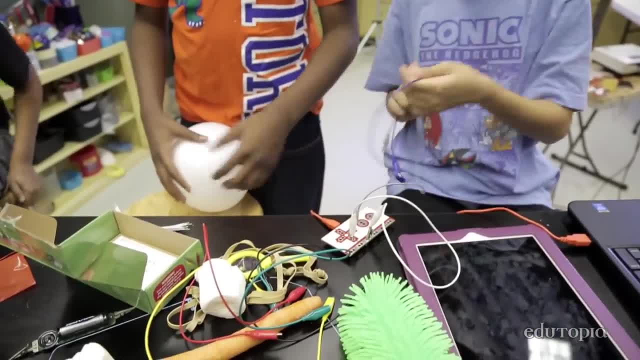 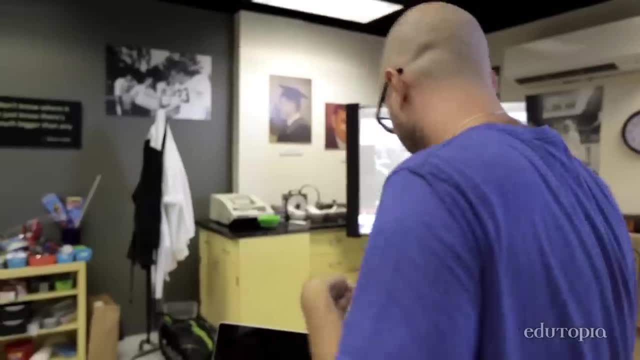 that's how inventors think. That's how artists who push the limit think. It's the same as how scientists make new discoveries. Scientists don't think of the scientific method. They're trying to push what's possible. So I'm going to start by taking a piece of some tofu that I was just eating. 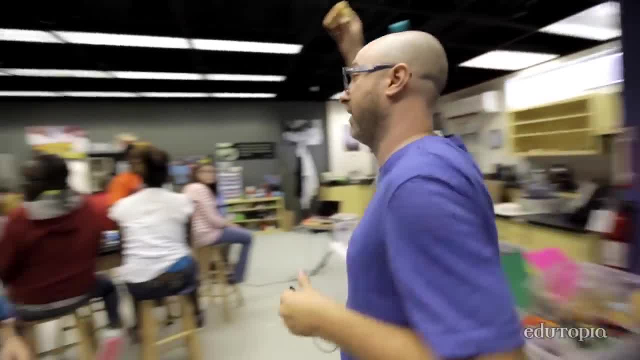 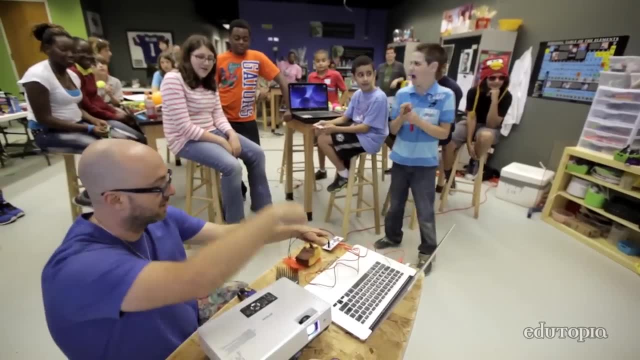 Oh, actually I ate all the tofu. I'll have to take the cornbread. So you hook up the cornbread to one of these four buttons or one of these spacer clicks, So I'm touching the cornbread. the video starts. 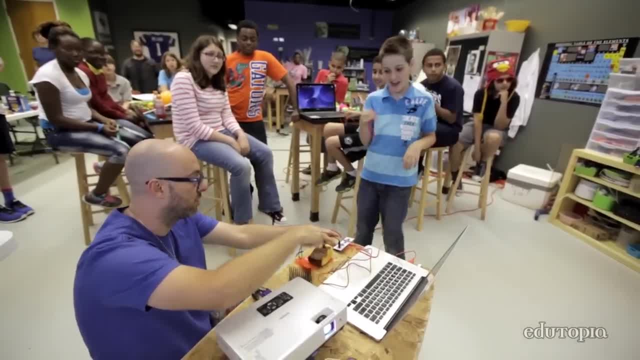 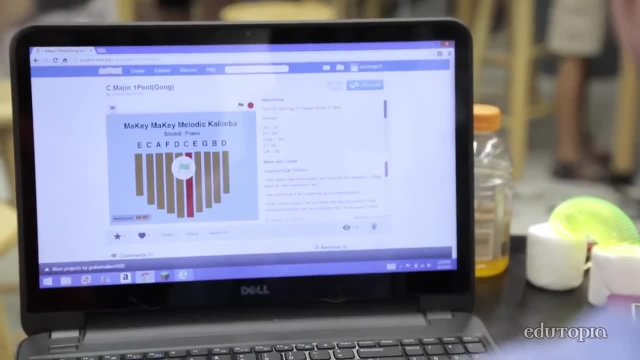 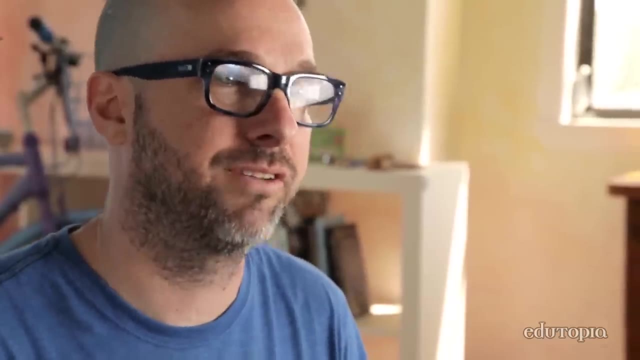 I touch it again, the video stops. If you take everyday supermarket stuff and you give a catalyst- in this case you know, electronic duct tape, like a Mickey Mickey. you have just changed technology, changed everyday objects and now you have changed yourself because you have this creative confidence. 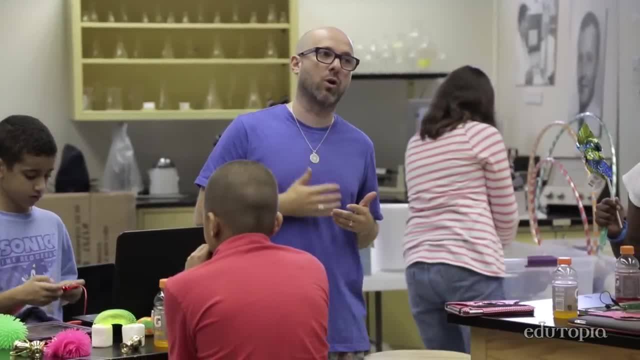 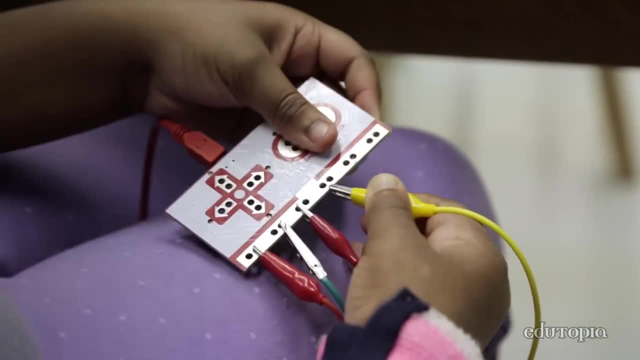 that comes from this experience. Over the next 90 minutes, we're going to work towards making an invention. You're going to make you know stairs into a piano, or you're going to make your bench into a Pac-Man controller. 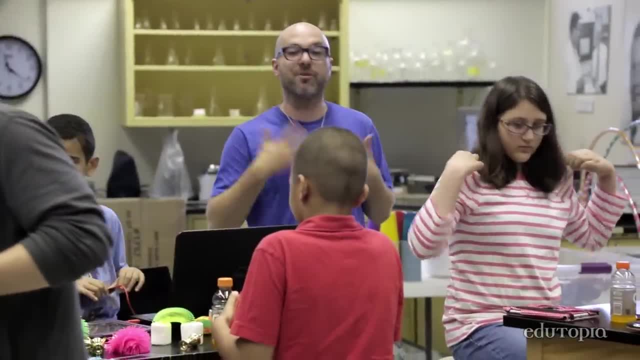 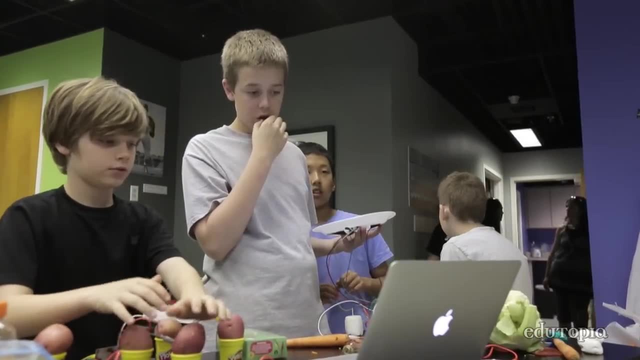 or you're going to take a book and when you open it it's going to send an email. Something's going to happen when you touch something. You might ask: is this about making a scientist or is this about making someone who's resourceful? 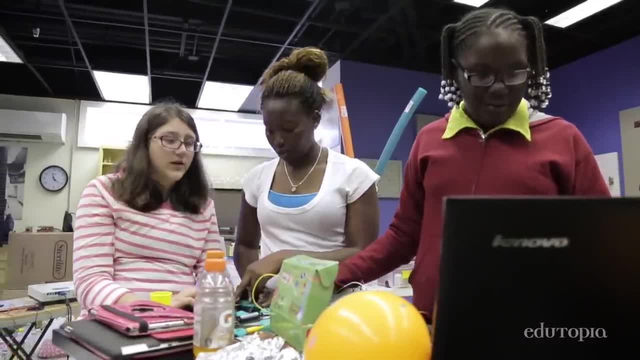 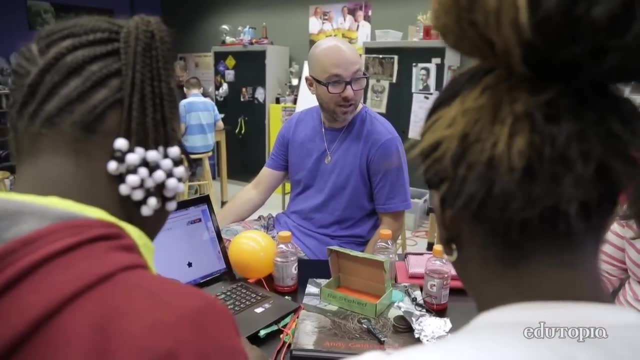 and can address problems in multiple ways. Well, I don't think there's any difference between those two questions. What are you guys working with over here, Having trouble making it work? Oh, what kind of troubles. I think people have the wrong idea of what scientists do. 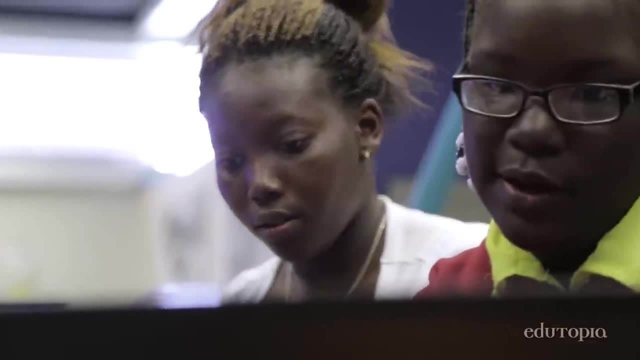 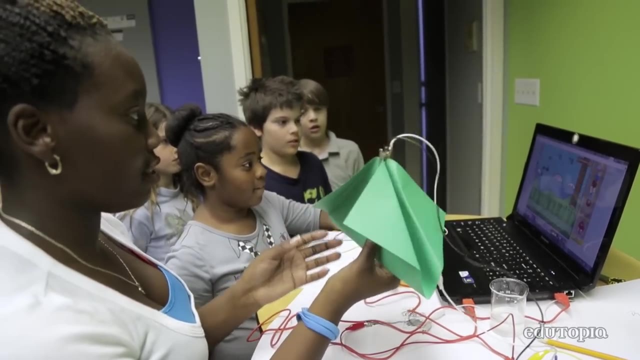 A scientist is a resourceful person who keeps attacking problems and fails 99 times out of 100. It's like a bird. Since I'm playing Flappy Bird, it's like a bird. I see there's two people playing at the same time. 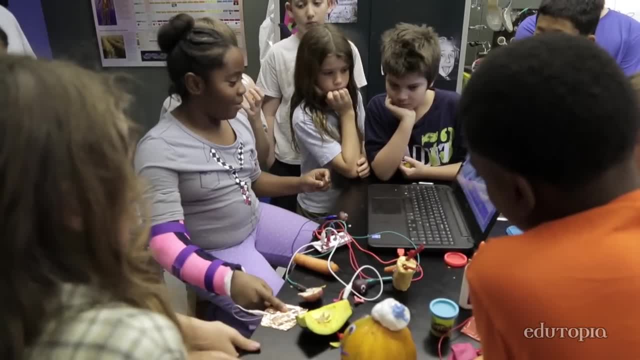 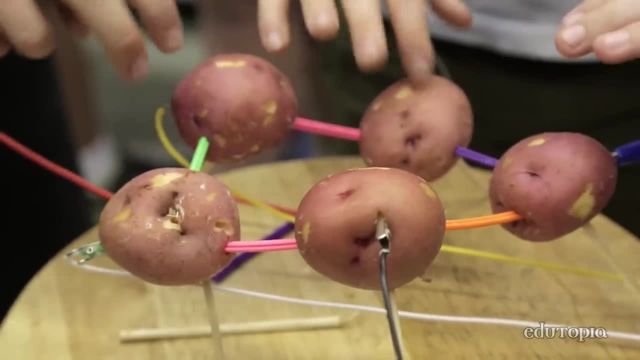 Mm-hmm, Smash it once. Hello, I'm Mr Fante, You're the good one. I'm Laura. This is up, this is right, this is left and this is down. Let's go, dance, Dance Revolution. 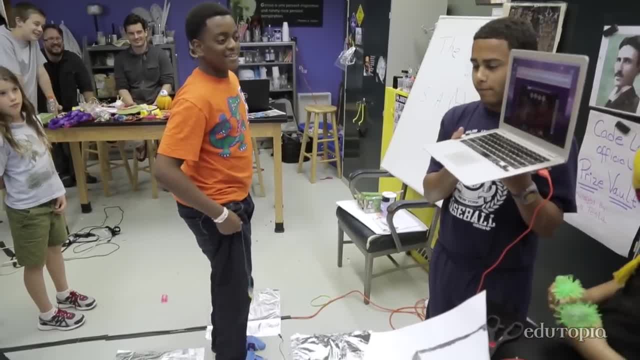 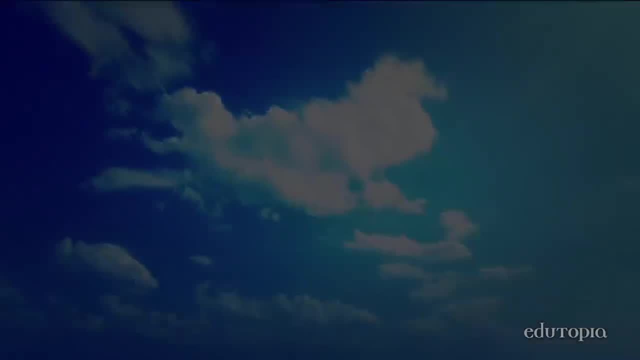 I'm not that good, so don't laugh at me. If a kid comes to you with a question, to assume that you have the answer is to assume that life is really simple. but it's not true. If a little kid comes to you and asks you: why is the sky blue? 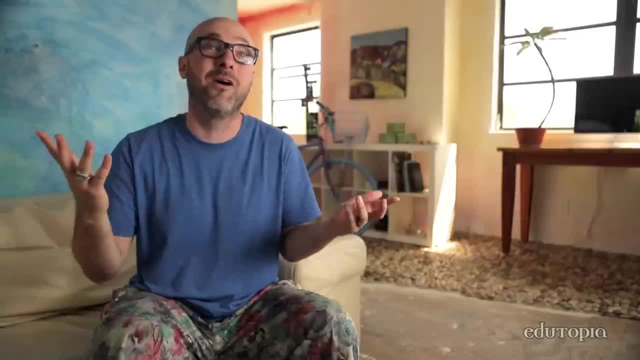 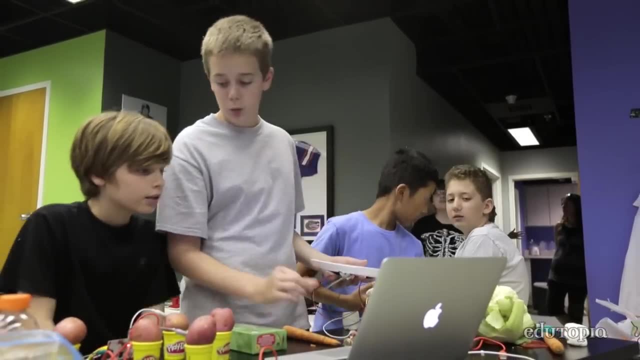 you may know something about scattering of light, You may think you know that it reflects off the ocean, but all of that doesn't matter. The point is it's about the process of them being curious. So don't try to give them answers, try to give them curiosity.